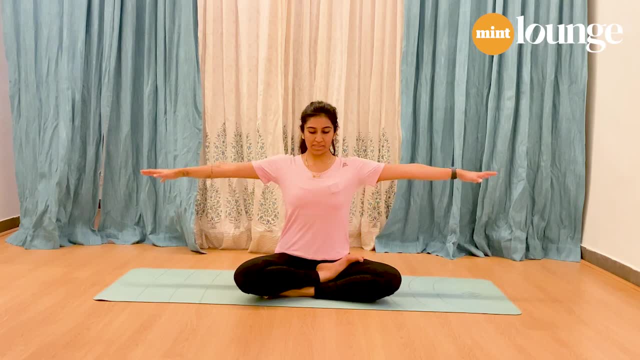 breathe deep into your chest and lift your arms up from the sides. Interlock your fingers and stretch up and feel your ribs lifting up nicely. Relax your shoulders and let's stay here and breathe For five every inhalation. lift the chest up more Four. 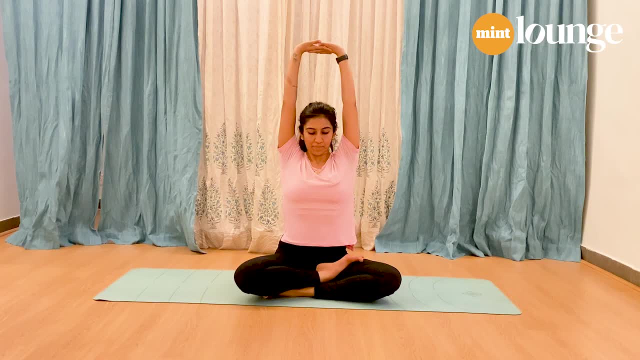 three, two and one. As you exhale, slowly bring your arms down. Next inhalation, lift your arms up from the sides. Interlock the fingers stretch up. keep the spine lengthened always As you exhale. you're going to bend your elbows and just drop. 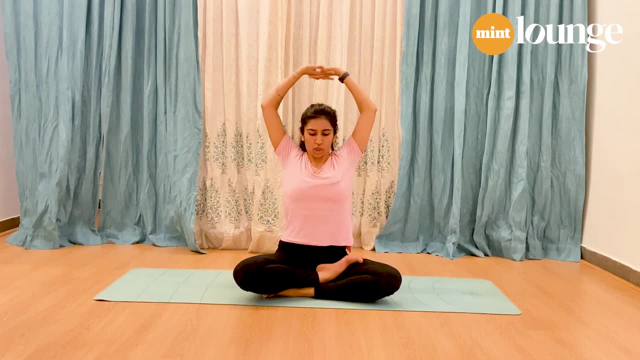 your palms behind the head. Your palms are still facing the ceiling. Drop it as low as you can and keep pushing your elbows As you exhale. you're going to bend your elbows and just drop your elbows out, Lifting the chest up nicely, opening up your chest from the sides. Stay here and breathe. 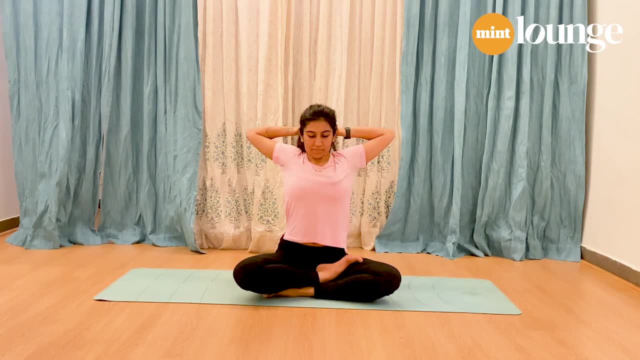 Five, four. breathe into the chest, Allow it to open up. Three, two and one, Exhale and slowly bring your arms down. Next one: you're going to open up the chest using your arms. I'm just going to show it to you from. 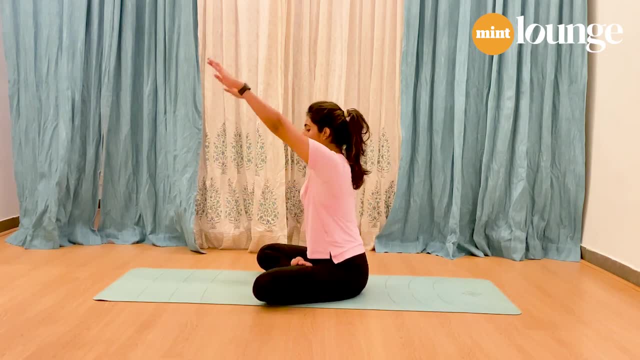 the side As you inhale, you're going to lift your arms forward and gently push your chest forward Slightly. lift your chin up. Stay here, breathe, Feel your shoulder blades coming together, Lift up. Stay here for five, four. 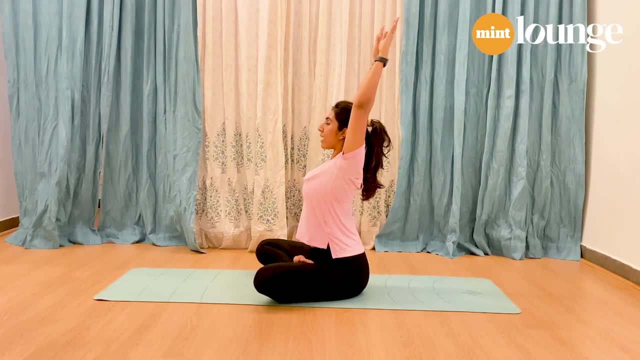 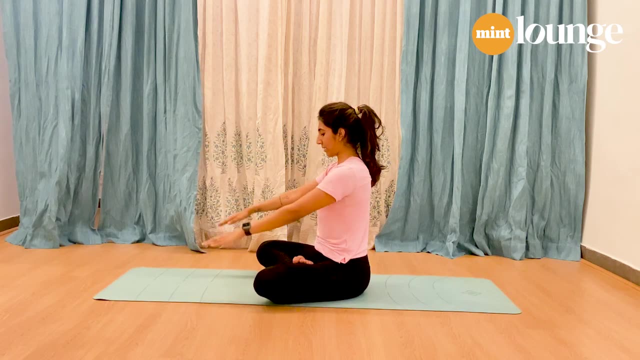 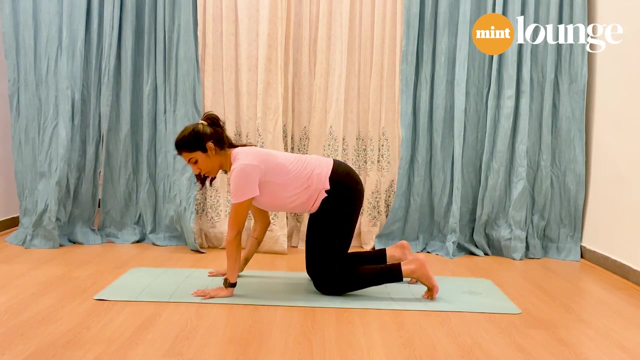 three, two and one. Exhale and slowly relax, Release your legs and come onto all fours. You can use cushions under your knees if you need to. if your knees are bothering you, Your wrists are in line with your shoulders, knees in line with the hips. As you inhale, you're just going to drop your hips. 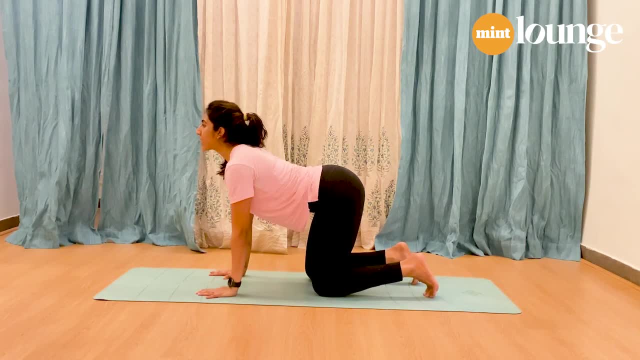 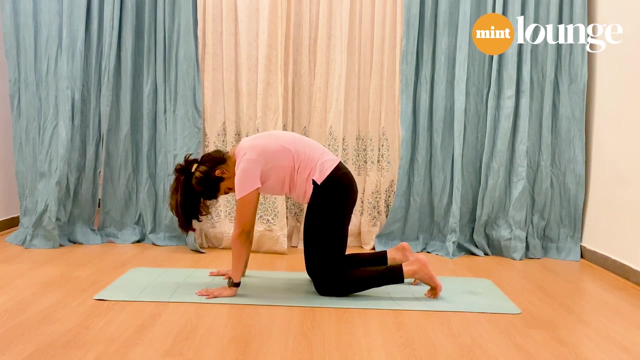 open the chest up. Exhale. draw your abdomen in. Drop your chin down, Round your back. Inhale- arch your back and look forward. Exhale around the back. Inhale- arch your back, Look forward. Stay here and breathe. 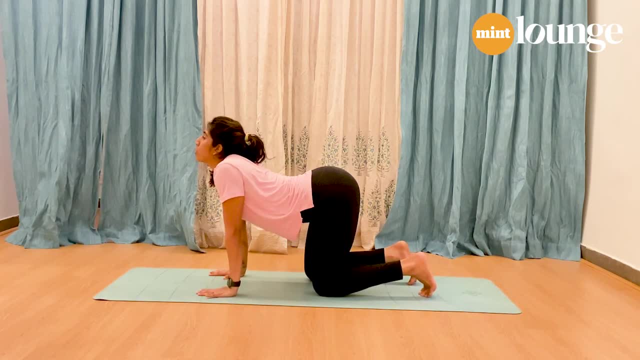 Make sure your chest is open and you're not sinking into the shoulders. Push away, Stay here, Breathe for five, four, three, three, two, one. Draw your abdomen in, round your back, chin down. stay here for five, four, three. 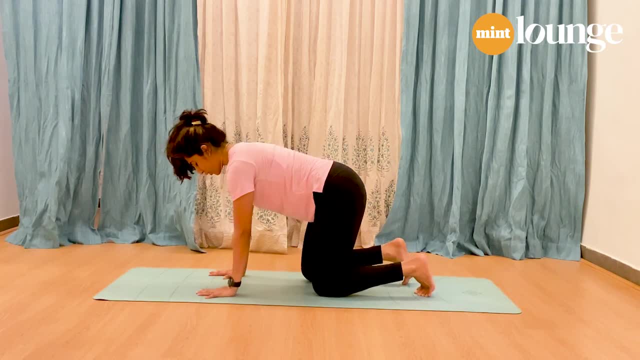 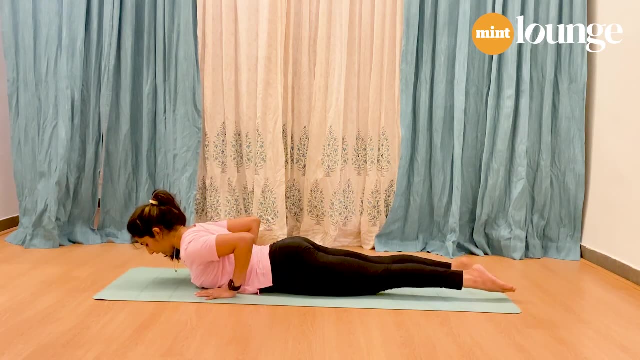 two and one. Come back to neutral. stretch your legs. lie down completely on your mat. try and keep your feet together. if that's uncomfortable, you can keep your feet hip width apart. your palms are right near your chest. elbows into the body forehead down on the mat. 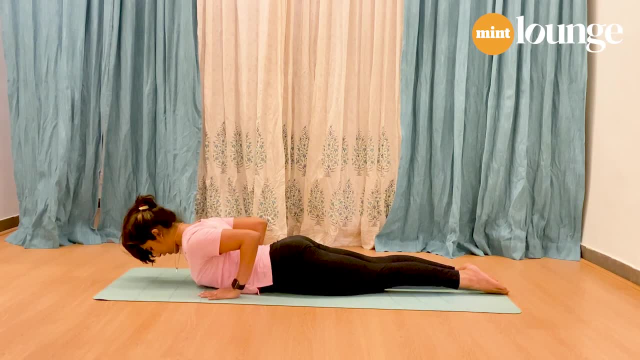 as you inhale, you're going to lift your head up, chest up. try not to straighten the elbows, just stay comfortably away from the mat. exhale slowly, come down. shoulders are always away from the ears. inhale- lift the chest up. 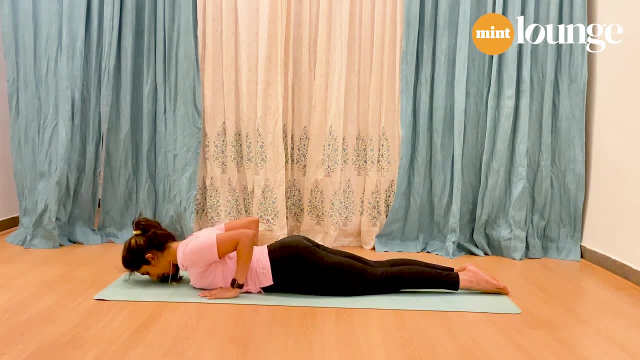 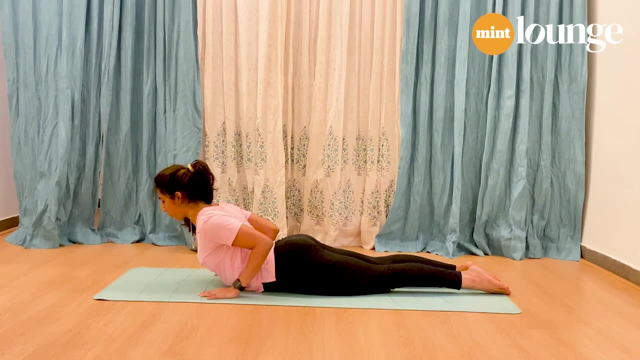 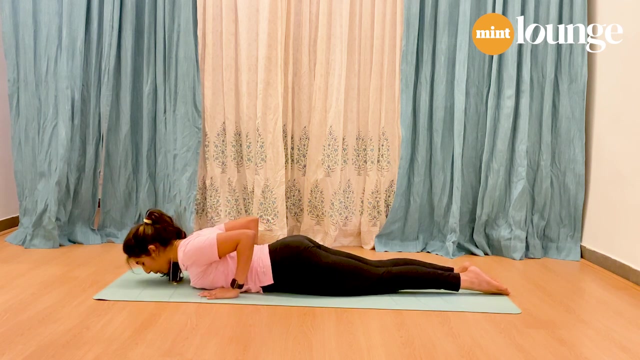 exhale down, inhale, lift the chest up. five, four, three, two, one exhale down. If you are very comfortable doing this, try to interlock your fingers behind the back, straighten your elbows, inhale, lift the chest up, stay here. five. 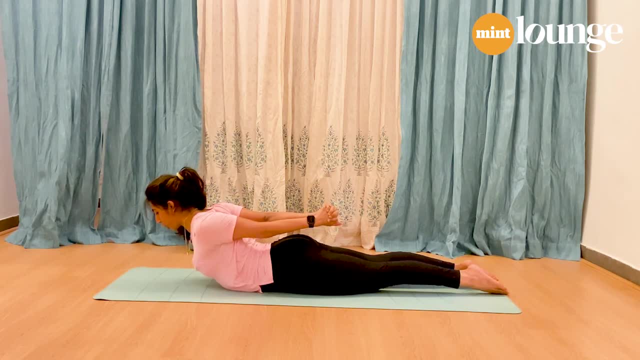 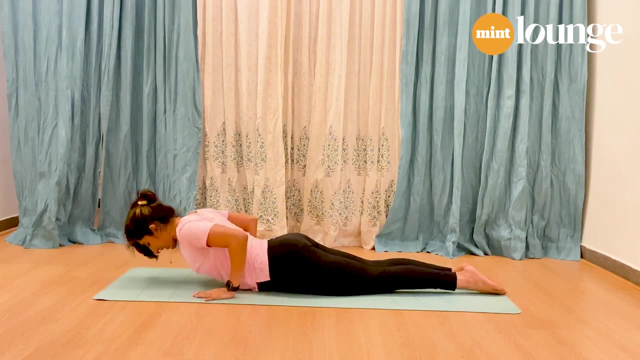 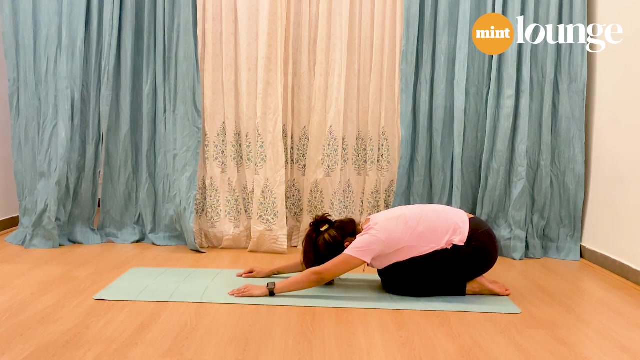 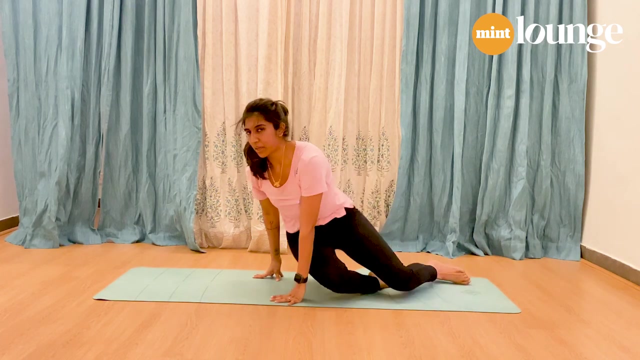 four, three, two, one exhale. slowly come down, bring the palms near the chest exhale. sit back in balasana or child's pose. allow your back to relax. slowly, roll up and come back to a comfortable cross leg posture.